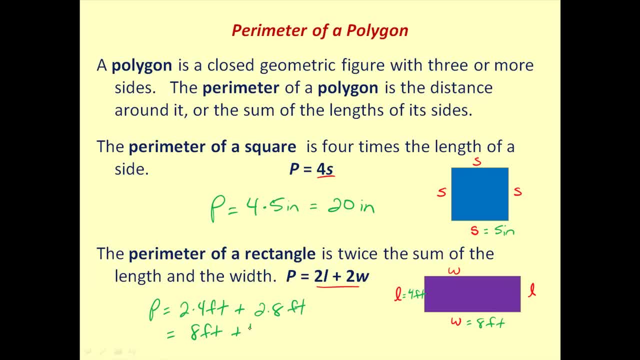 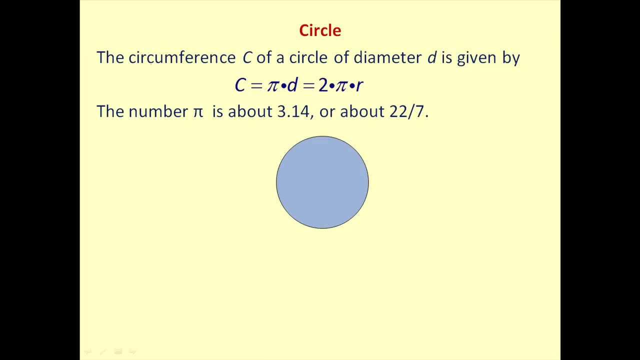 Which would equal eight feet plus sixteen feet, Which would give us a perimeter of twenty-four feet. So if we find the sum of the lengths of all four sides, we would get twenty-four feet. Now let's talk about a circle. The perimeter of a circle is called the circumference. 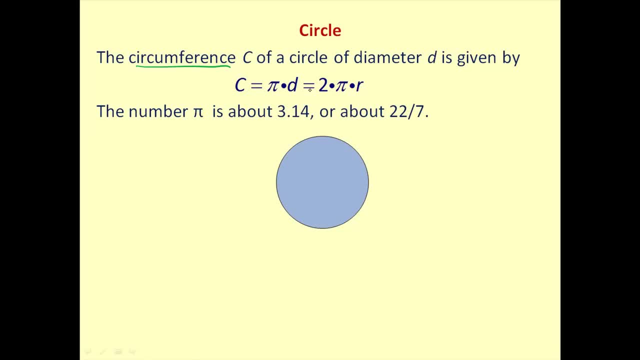 And the circumference is equal to pi times the diameter, or two times pi times the radius. The diameter goes from one side of the circle to the other, passing through the center, While the radius is a segment from the center to the edge of the circle. 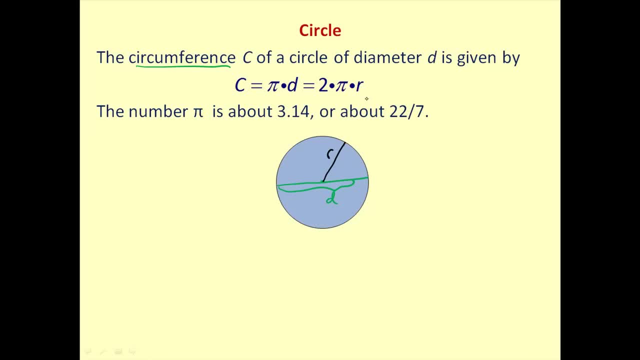 So, depending on what you're given will affect which formula that you'll use. However, if you look at this sketch, If you multiply the radius times two, it would equal the diameter, Or you can say that the radius is half the diameter. So, as an example, if we were given that the diameter is equal to twenty meters, 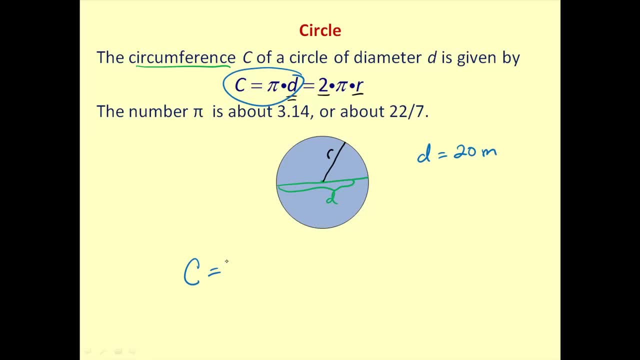 We would use the first formula, And that would be pi, Which is approximately three point one. four Plus twenty meters, Which would equal sixty-two point eight meters. Now, this is approximately equal to pi. So this is an approximation of the true circumference. 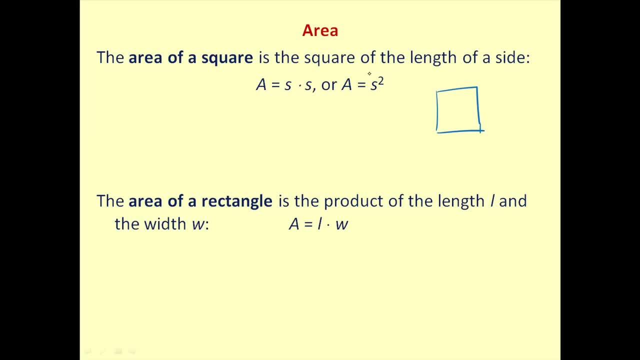 Okay, let's go ahead and talk about area now. The area of a square is the square of the length of a side. So again we know all of these sides have the same length, If we're given that this length is equal to four centimeters. 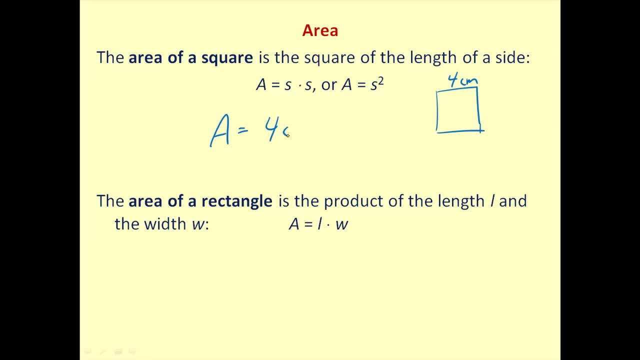 Then the area will equal Four centimeters times four centimeters, Which will equal sixteen centimeters squared. Notice: the units for area are square units And where that comes from is if we were to take this square And divide it into square centimeters. 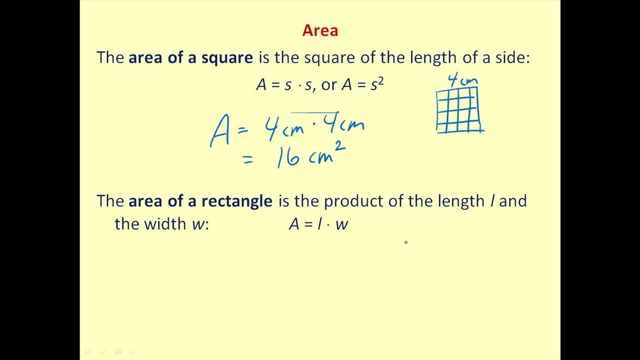 There would be sixteen of them inside the square And this is very similar to a rectangle. If I have a rectangle that is five millimeters by eight millimeters, The area will be equal to the length times the width, Or five millimeters times eight millimeters. 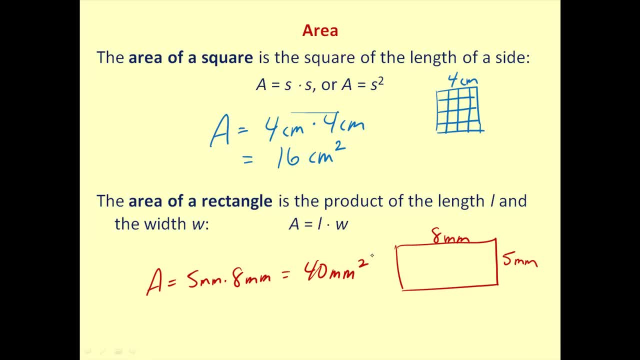 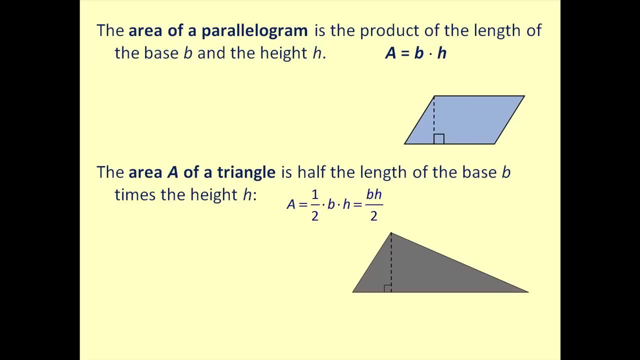 Which would give us forty millimeters squared. Now let's talk about the area of a parallelogram. The area is the product of the length of the base and the height, Or the base times the height. So this is the base. So if this base is equal to twelve meters, 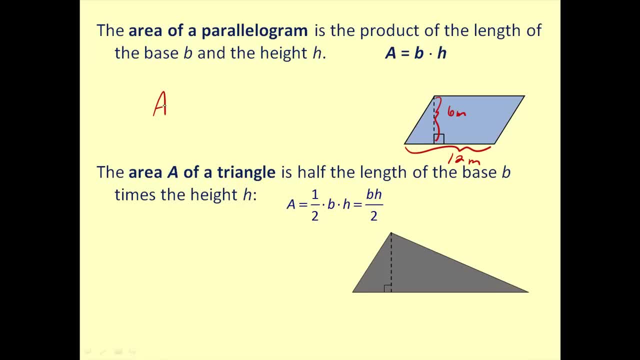 And the height is equal to six meters, Then the area is equal to Six meters times twelve meters, So seventy two meters squared, Which is just like the area of a rectangle, Because if you take this triangle and you put it over here, 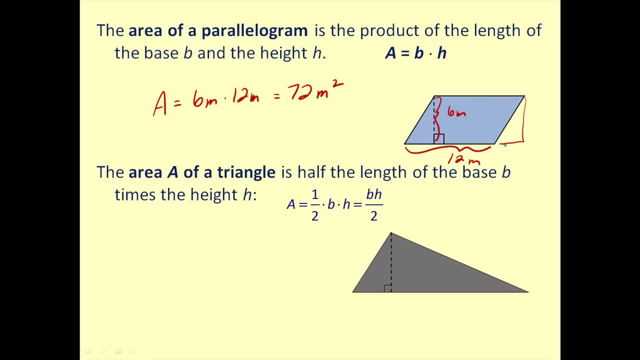 You would have a rectangle, But we'll take a look at that in more detail at the end And next We have the area of a triangle. The area is half the length of the base Times, the height, Or base times height, divided by two. 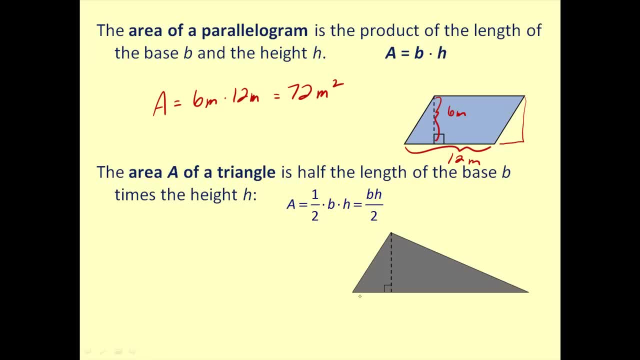 Remember, dividing by two is the same as multiplying by one half. So again, here's our base. Let's call this Twenty feet And our height, Let's say, is eight feet. Then the area is equal to. I'll use the second formula. 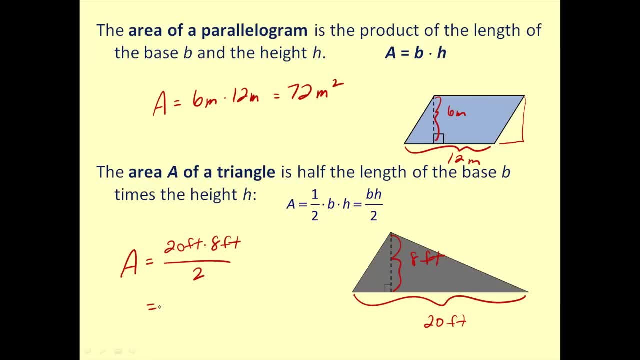 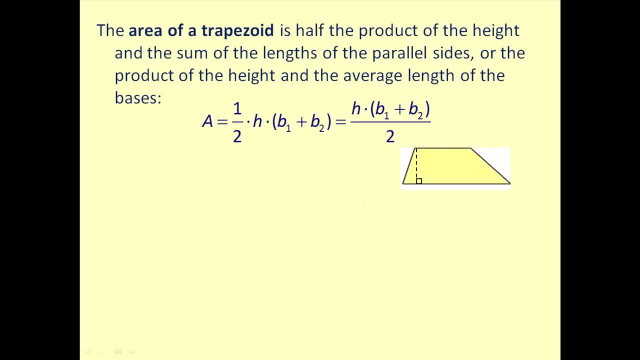 Base times the height Divided by two, Which equals eighty square feet. Let's move along to what's probably the most involved area formula. It is the area of a trapezoid. The area is equal to half the product of the height. 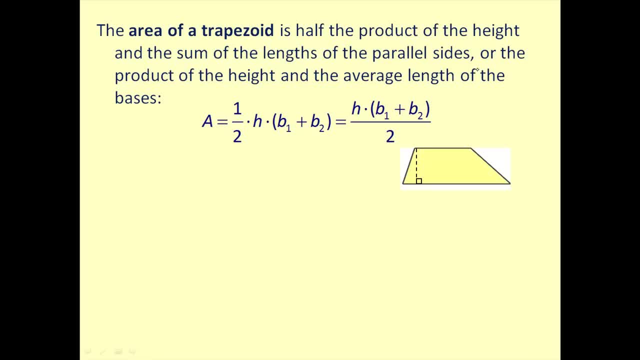 And the sum of the lengths of the parallel sides, Or the product of the height and the average length of the bases. This would be base one, This would be base two And, of course, this is the height. So, as an example, If this is fourteen inches, 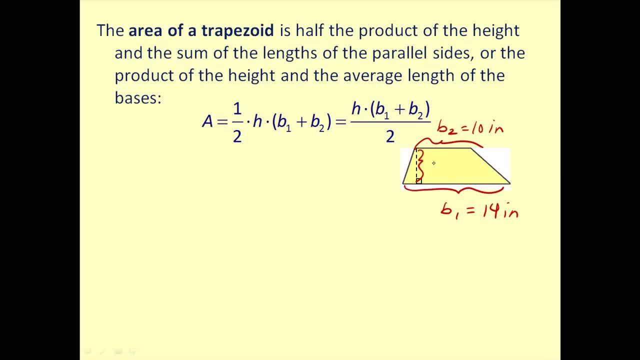 And this is ten inches, And our height is equal to six inches. Let's go ahead and use this first formula this time. The area is equal to one half Times the height of six inches, Times The sum of base one plus base two. 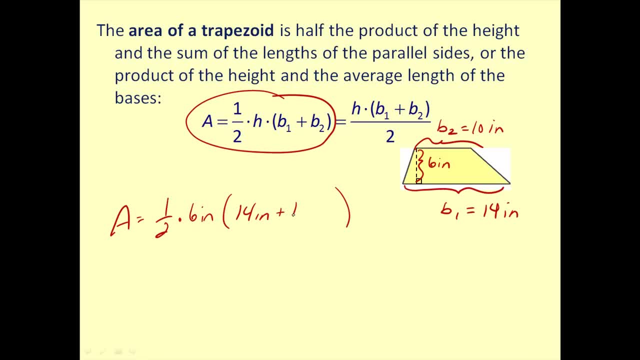 Or fourteen inches Plus ten inches. Now notice how I'm leaving the units in the formulas. A lot of times textbooks don't do that, But I like leaving them in because it really reminds you that area is in square units And the perimeter is not. 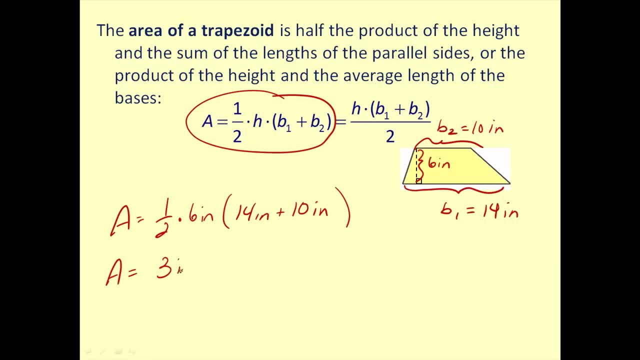 So here we have one half times six inches, That would be three inches. Fourteen inches plus ten inches equals twenty four inches. You can see we have Three times twenty four, That would be seventy two, And inches times inches Is equal to inches squared. 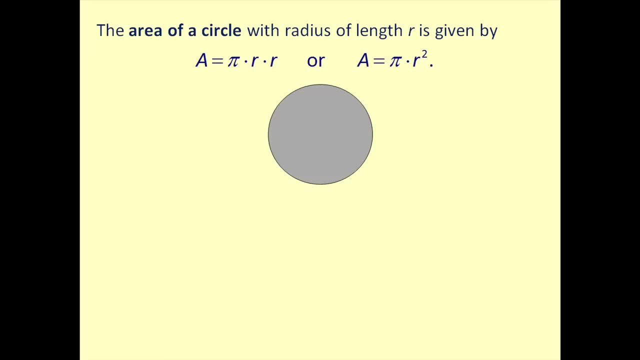 The last formula we'll look at Is the area of a circle. Notice the area formulas for a circle involve the radius. So if you have the diameter, You do have to divide by two to find the radius for this formula. So area equals pi, times radius, times radius. 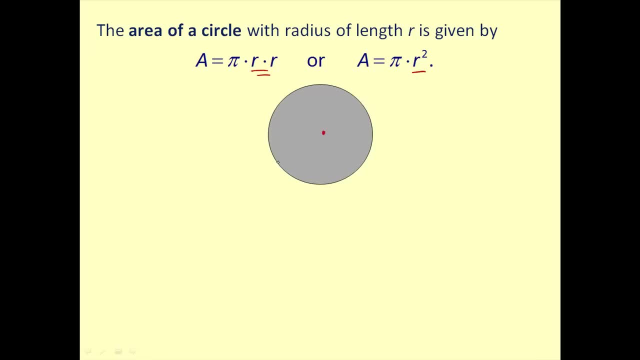 But of course this can be written as r squared. So if we're asked to find the area Of this circle, The first thing that they recognize is We need the radius. This is the diameter, So the radius would be half of that, or five feet. 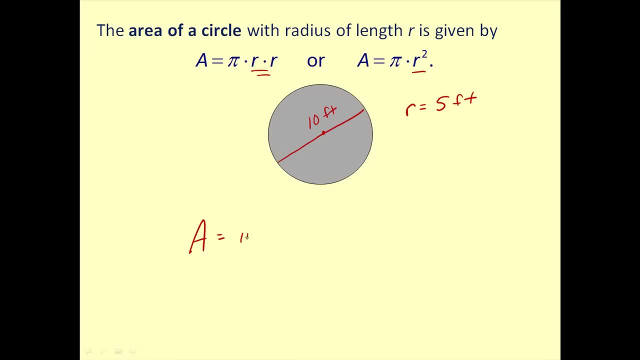 So the area is going to equal Pi Times Five feet squared, Which would give us twenty five pi Feet squared. Remember, pi is a constant, But normally we do want to get a decimal approximation of this. If we multiply twenty five times three point one four: 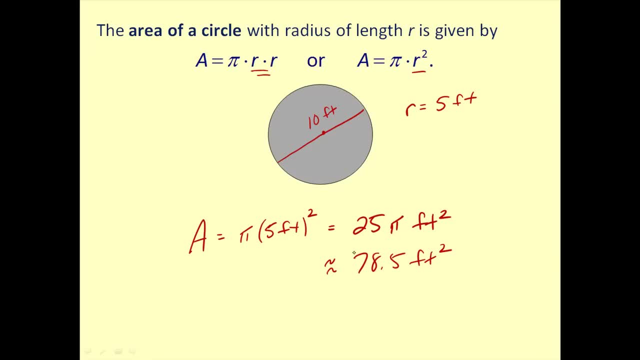 We get Seventy eight point five Square feet. Notice it's approximation. Okay, let's go ahead and take a moment And see where these formulas actually come from. I would highly encourage you to visit this website And do some of your own exploring. 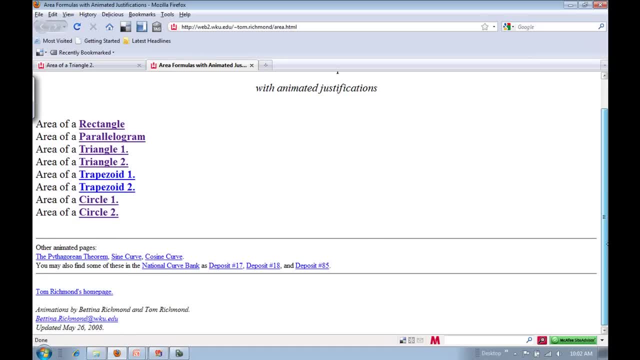 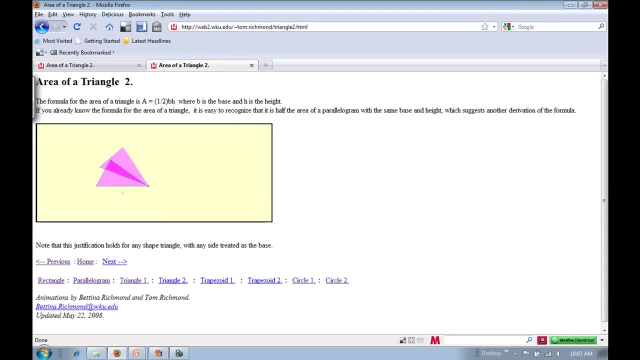 You have the website, And these were made by Bettina and Tom Richmond. Let's go ahead and take a look at this triangle Animation. So what happens here is you double the triangle And then you slide it To form a parallelogram. 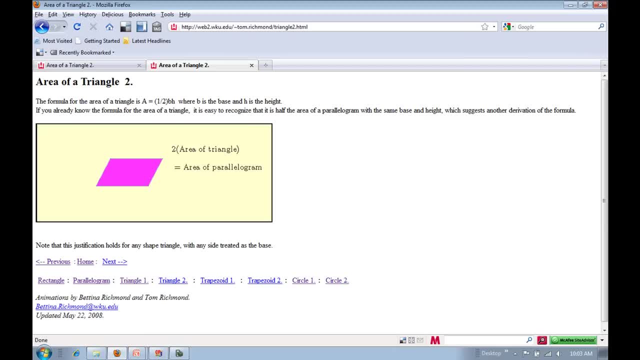 And we know that the area of a parallelogram is base times height. So if we take the area of this parallelogram and then divide by two, You would have the area of the triangle that we're looking for. Let's go ahead and take a look at the parallelogram also. 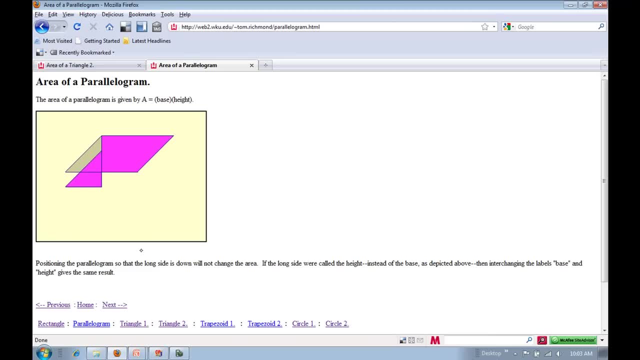 So what we do is we draw an altitude, creating a triangle, And then we move this triangle over to the right side And you can see now It has the same area as a rectangle And the area would be base times height The same as a rectangle.